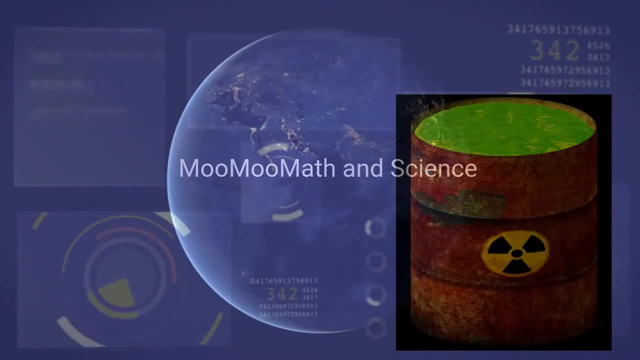 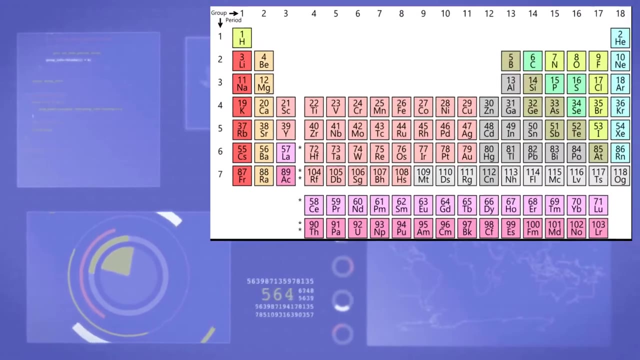 Welcome to MooMooMath and Science. In this video I would like to talk about the radioactive elements, or the actinide series of metals. When you look at a periodic table, many times you will see rows 6 and 7 at the bottom of the periodic table. This is done in order. 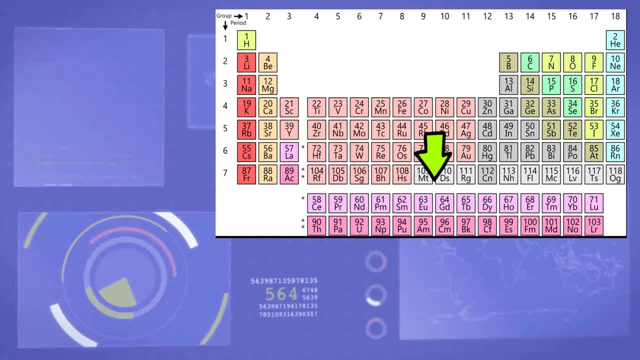 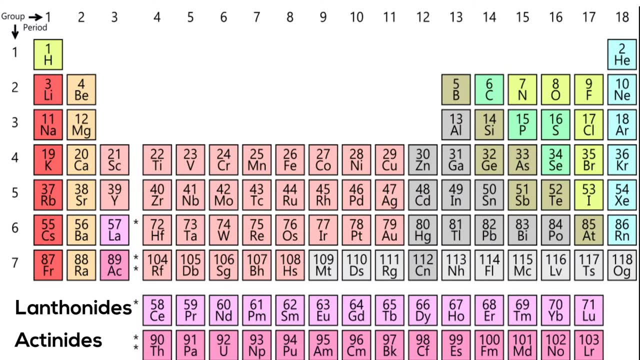 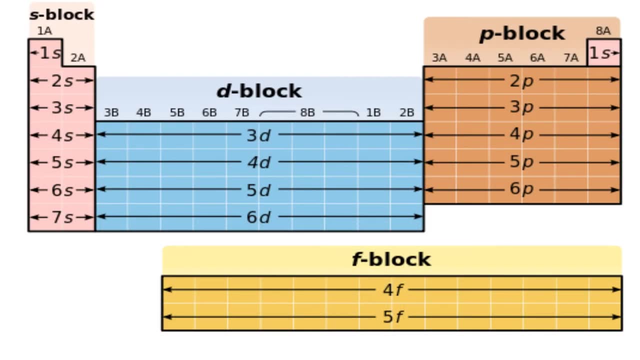 to keep the table from being too wide. These two rows are called the lanthanide and the actinide series of transition metals. The actinide metals are found in group 3 and period 7.. These two rows are produced when electrons are added to the F-block orbitals. Therefore, 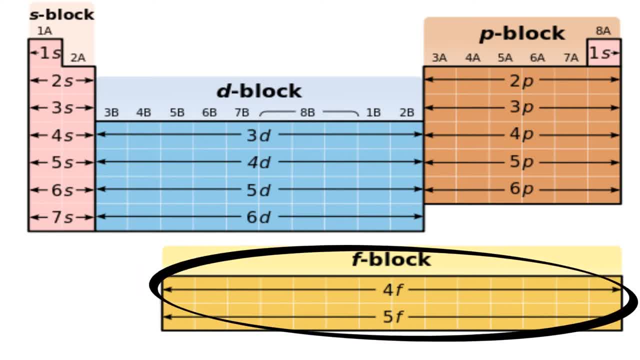 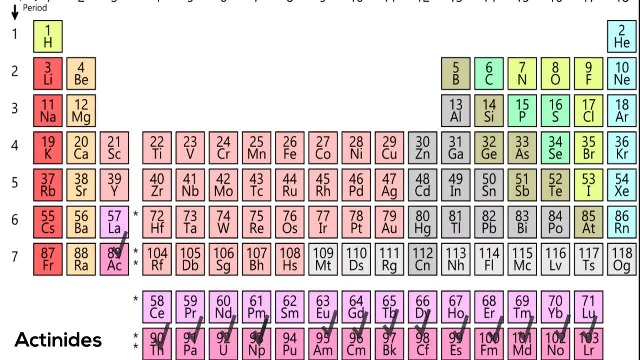 this block of elements are referred to as the F-block elements. The actinide series of metals make up the 5F-block. The actinide metals are elements 89 through 103 and are transition metals. The actinide elements are radioactive and unstable. Elements listed after plutonium. 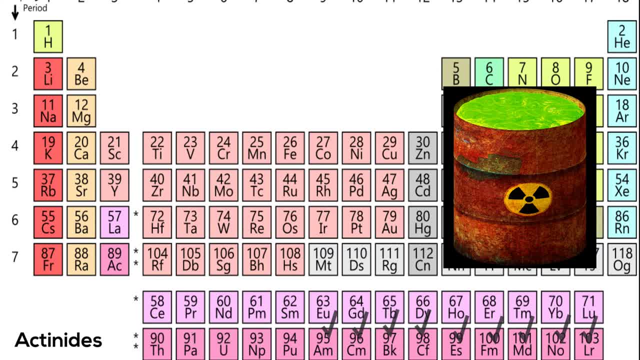 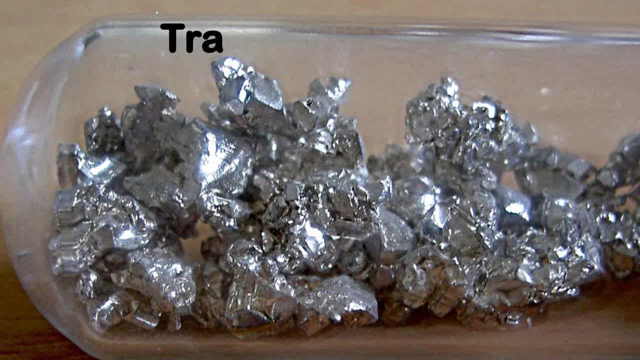 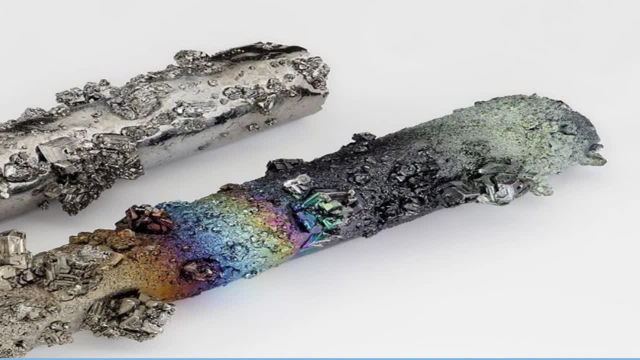 which is element 94, do not occur in nature and have been made in the lab. The actinide elements have the following properties: They are metals, They are radioactive, They tarnish easily in the air and are very dense and have the ability to combine with most non-metals. You can see that the actinide elements are radioactive and unstable. The actinide elements are radioactive and unstable. The actinide elements are radioactive and unstable. They are radioactive and unstable. They are radioactive. The actinide elements are radioactive and. 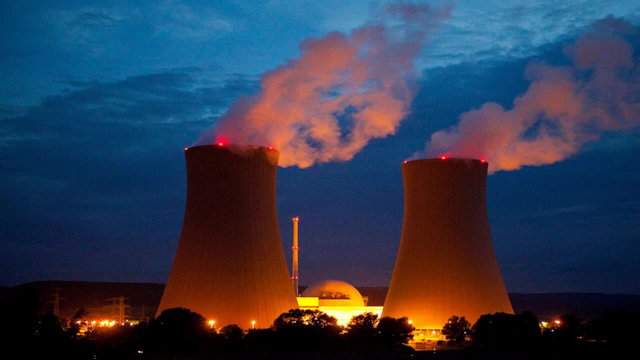 unstable. The actinide elements are radioactive and unstable. The actinide elements are radioactive and unstable. Uranium and Plutonium are probably the most known because of their use in the nuclear industry and in the military. Here's a list of each actinide metal and a quick fact about it. 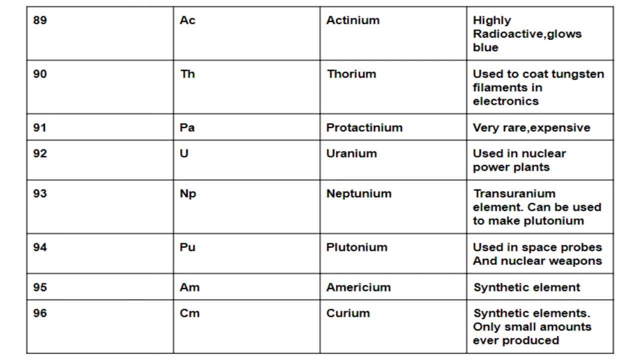 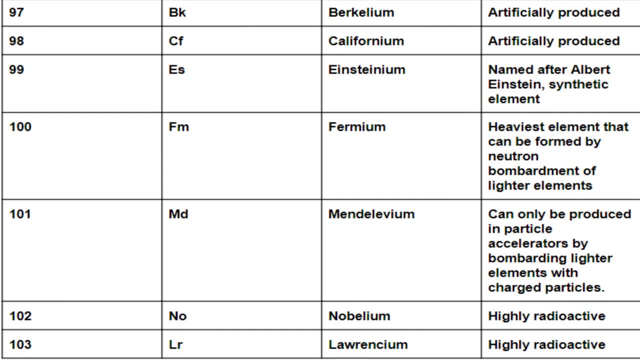 Here's a list of each actinide metal and a quick fact about it. Here's a list of each actinide metal and a quick fact about it. So there we go, that actinide metal, radioactive metals that are helpful and important war. thanks for watching and move mood math uploads. 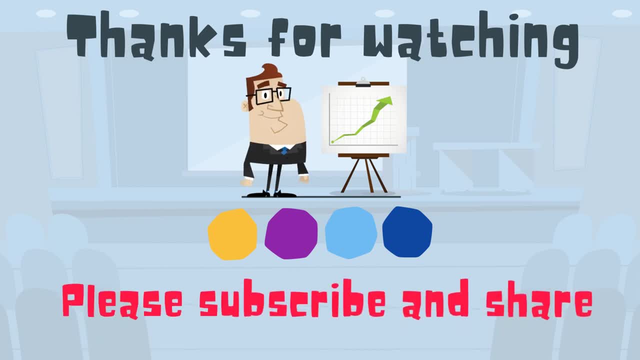 and effective metal that aren't radioactive metals. please subscribe and please be sure that you hit that. i notifiedon How to his atomized sub-eee. j να know about limiting builders video every day. Please subscribe and share.